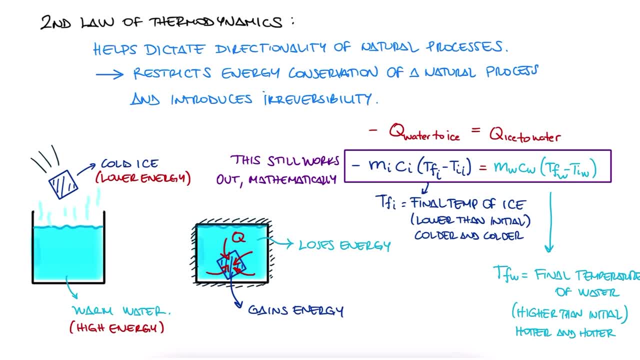 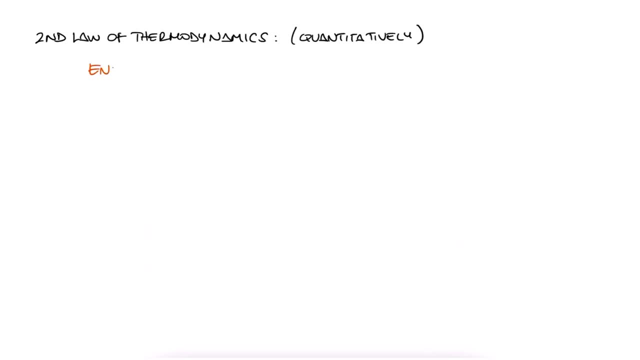 example. we don't need an entire law of thermodynamics to know that the second case is simply not physically possible, But in general, that is indeed what the second law does, at least qualitatively. One of the qualitative benefits that the second law of thermodynamics offers is related to the 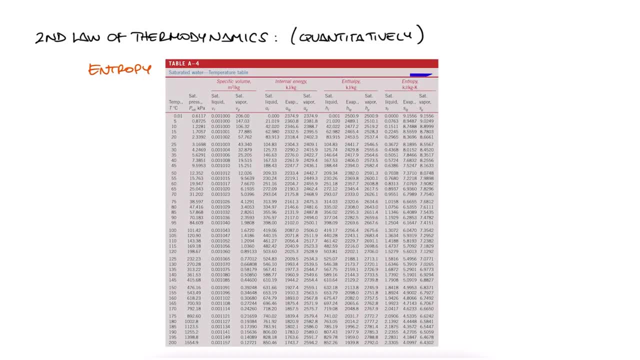 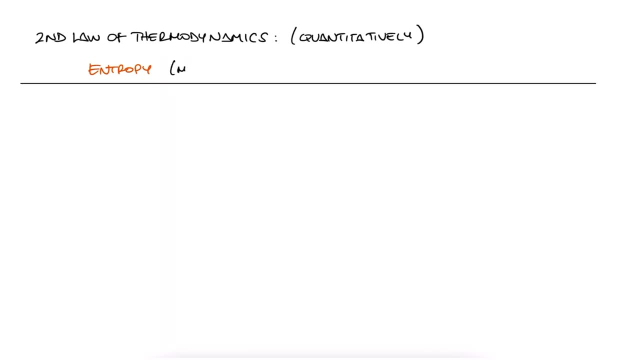 entropy. We've seen values for specific entropy S in some of our property tables, but we'll get to that later. Let's go back to the ice cube type examples. In a slightly less obvious scenario- still very obvious, though- we know that we can, for example, add work to a tank with a fluid. 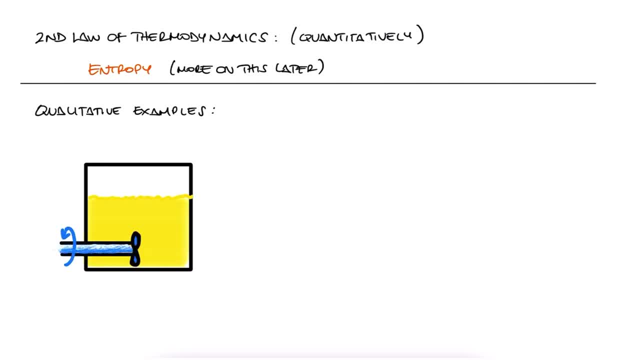 in the form of a rotating paddle wheel to make its contents heat up and have the system put out heat to the environment. From the first law of thermodynamics we know that the second law of thermodynamics offers heat to the environment In the first law perspective. we could very well say that we 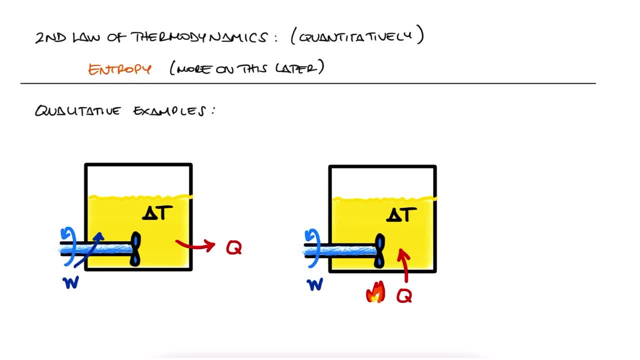 can do the opposite, that we can add heat to the fluid and extract work. But we know that this is not possible. Just because the contents of the tank are becoming hotter, the paddle wheel is not going to start rotating spontaneously, And this is easily seen with the help of the second law. 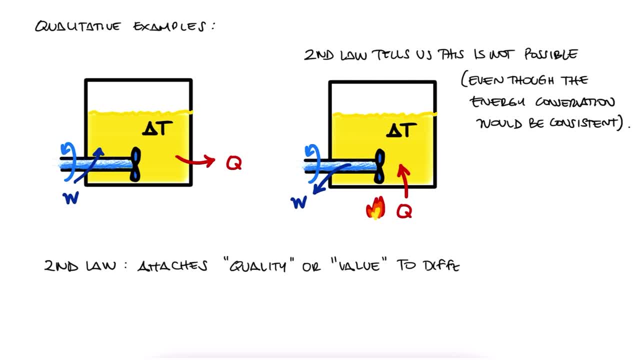 The second law attaches a quality or value to the different types of energy. When looking at different types of energy from a first law perspective, we don't care if it's the thermal or work or kinetic energy. they're, in practice, interchangeable. The second law actually. 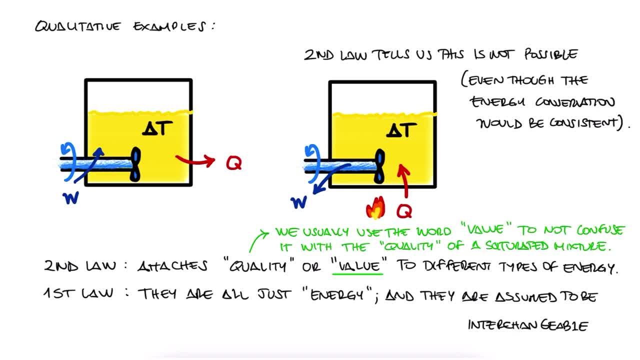 tells us which one has a higher quality or value. So with this example of the paddle wheel, we understand that a single process can be irreversible. However, we can have a similar situation where, in practice, we can in fact extract work out of adding a heat to a system. 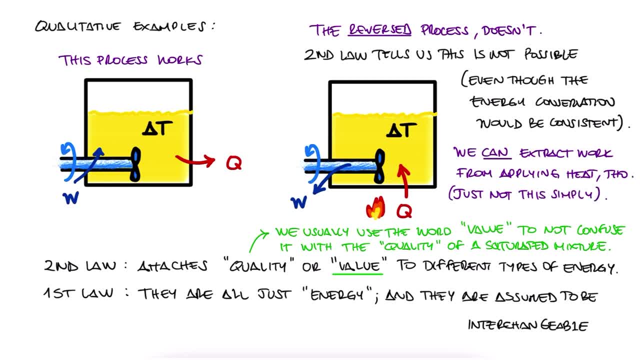 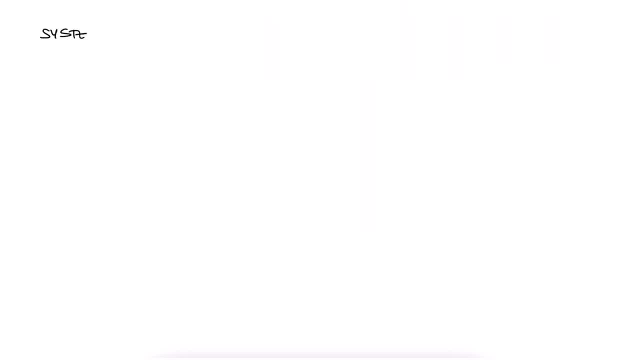 So we'll come back to the second law of thermodynamics in much more detail later, two lectures after this, one link below. But for now we'll focus on a couple of particular systems where we can engineer our way into turning heat into work. For example, let's assume a closed system, a piston-cylinder system, where we bring 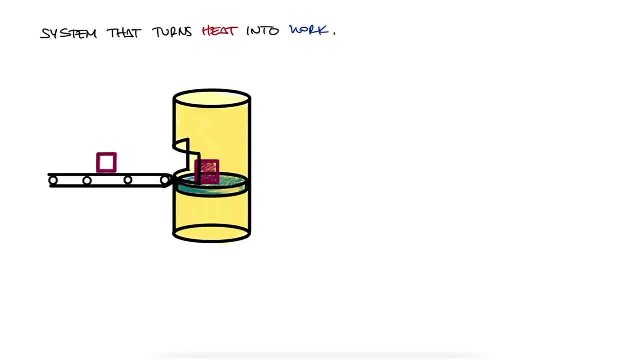 in a mass, let's say, the conveyor belt drops it at the top of the piston and by heating the gas inside of it, we bring the mass to a higher altitude. This is effectively using thermal energy to gain potential energy or, what is the same, to extract work from the system. 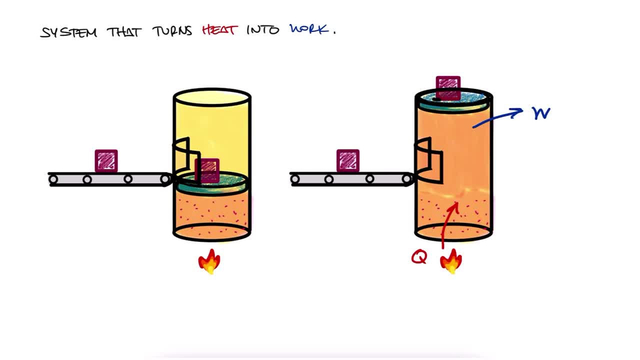 What if we want to start over? What if we want the piston to go back to its initial position, so that the next mass that is coming in from the conveyor belt can also be brought up using the piston? Well, we could cool down the gas inside the system. 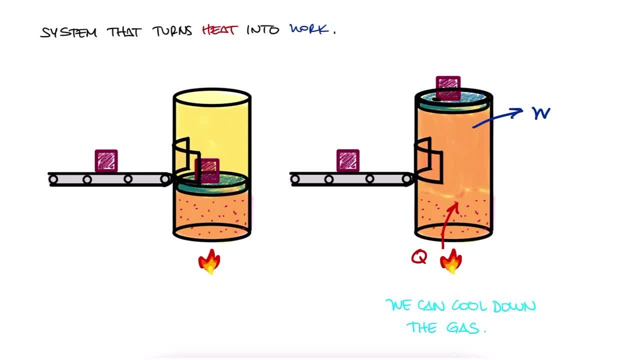 right, And this doesn't necessarily mean that we're subjecting the system to, let's say, a flame and then cooling it down by blowing on it. right, We can have a high temperature reservoir: provide the heat to the system in step one, and a low temperature reservoir take the heat from the. 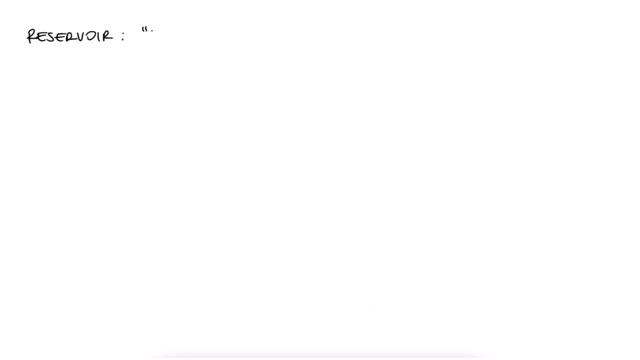 system in step two. The term reservoir is a system that can be used to generate heat from the system in step two. The term reservoir refers to a source so big that removing or adding energy to it will barely change its properties. If we have a drop of water that we add 10 joules of heat to the 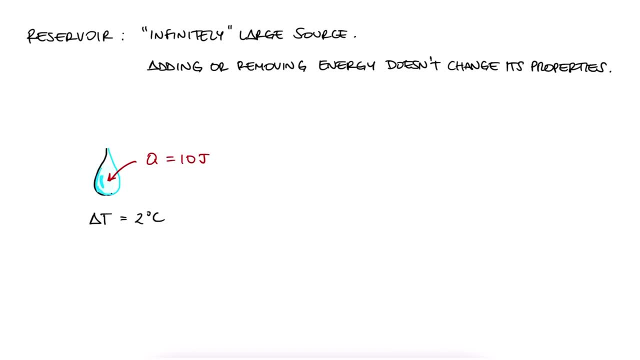 temperature of the drop will probably change by a couple degrees, But if we add 10 joules of heat to a lake, its temperature might just increase by so little that we wouldn't be able to measure it. In other words, reservoirs are sources that, in practical terms, 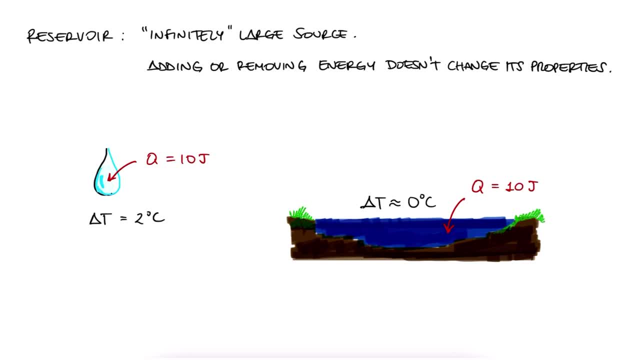 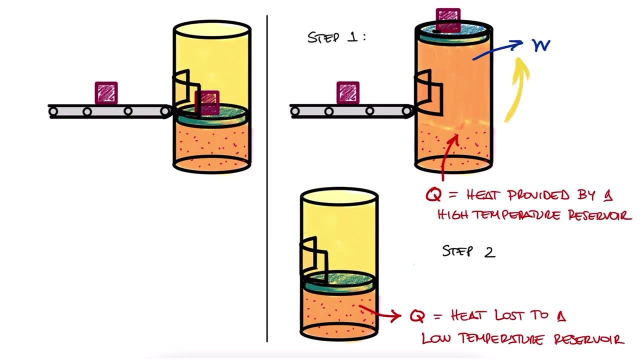 maintain their properties even when adding or removing energy from them. A system like this: add heat from a high-temp reservoir, extract some energy from it in the form of work and then bring it back to its original state by rejecting the remaining heat using a low-temp. 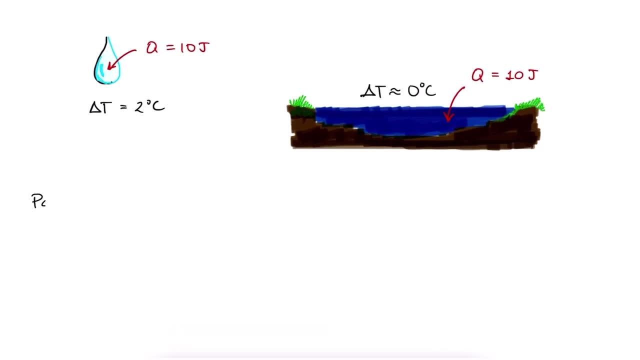 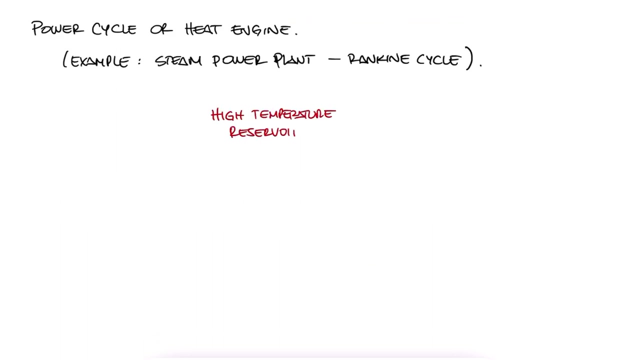 reservoir- and repeat this over and over- is what we call a power cycle or a heat engine. The most common example of a heat engine is a steam power plant, which operates on a ranking cycle. We'll learn more about this soon. In a steam power plant, we first have a high-temperature. 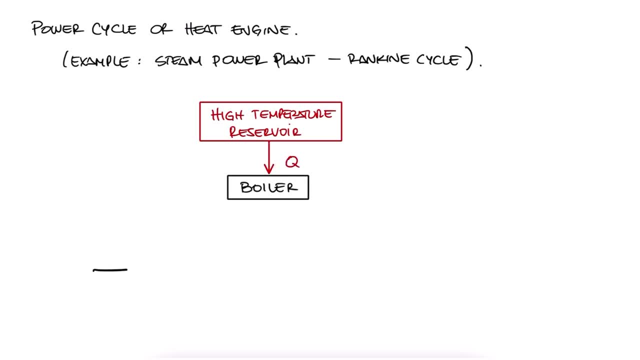 reservoir that supplies heat to a boiler. A boiler can be interpreted as simply as the pipe flow device we studied three lectures ago, link below. We have liquid water flowing through a pipe and we add heat to it to obtain steam. State 1 and state 2 would go before and after the boiler with no significant changes to. 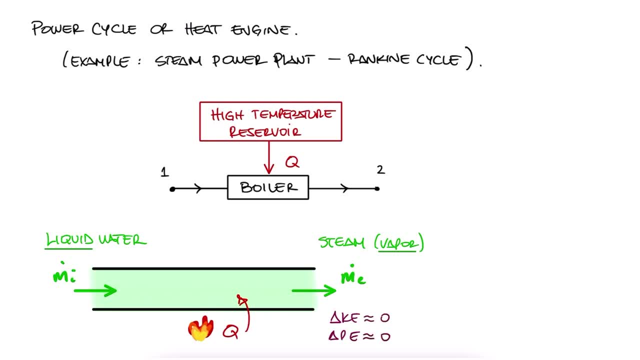 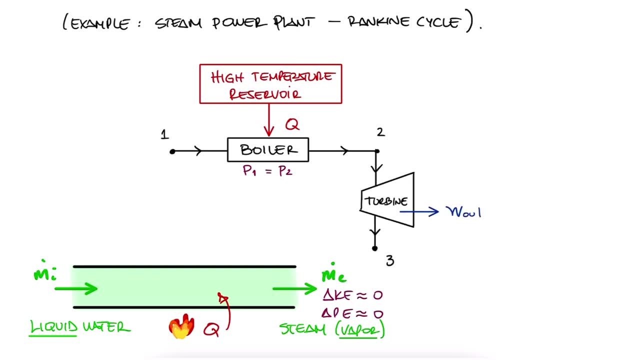 kinetic energy or potential energy, plus the assumption that the process occurs at a constant pressure. From 2 to 3, the steam goes through a turbine, which we already know allows a process to extract work, while decreasing the substance pressure and temperature From 3 to 4, we'll pass the fluid through a condenser. This condenser rejects heat to 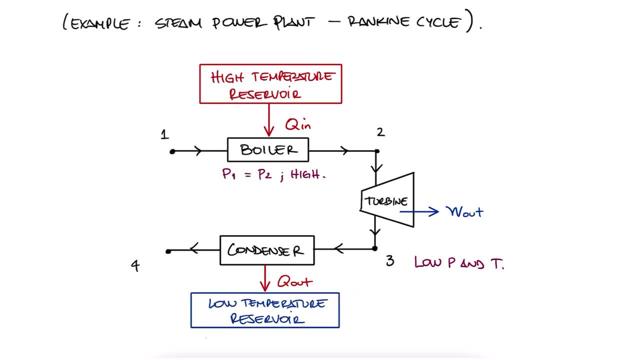 a low-temperature reservoir, and it can be considered as another pipe flow device where there's no significant changes in kinetic energy or potential energy and, just like the boiler, we keep the assumption that the process occurs at a constant pressure. only this time the constant pressure is a low pressure, as opposed to the pressure in the boiler. 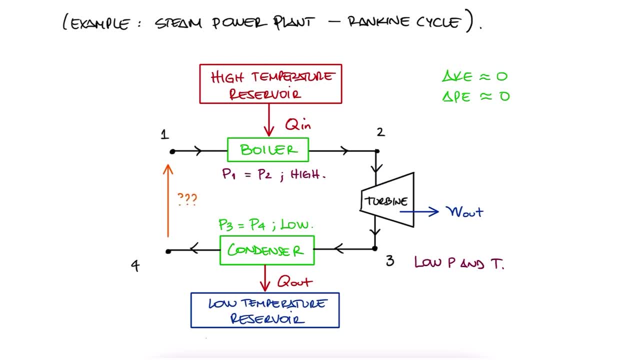 So how do we bring back the heat from the boiler? Well, we can do that by using a steam pump. The steam pump is used to pump the liquid back from state 4 to state 1.. Well, from the name that we're giving the second pipe flow device, the condenser, you can probably 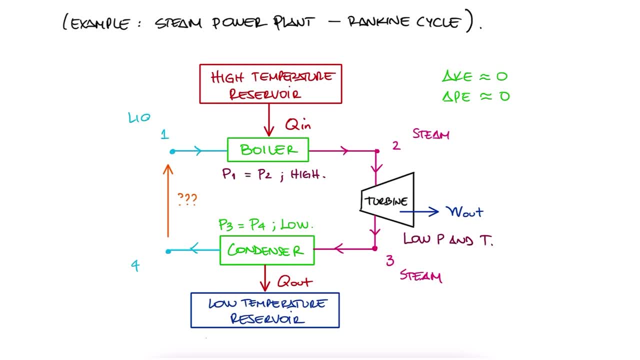 infer that that rejection of heat will allow the steam to go back to a liquid water phase. So if the main difference between states 1 and 4 is the pressure, we can bring it back up with another one of the steady-state devices we studied in the second lecture video of the 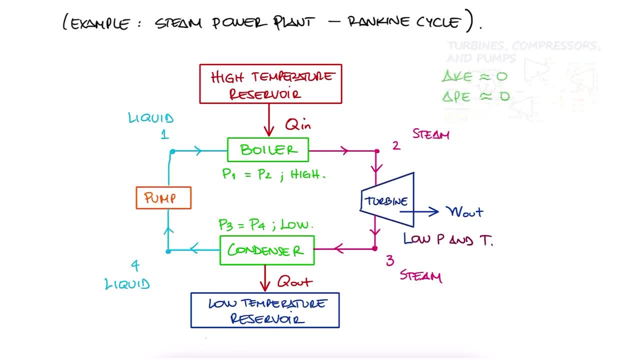 three-video series also linked below. That device would be the pump. Of course, this pump requires some work input to do. The pump requires some work input to do and that's why this cycle will have a net work out: The work we obtain from the turbine minus the work we need for the pump to operate. 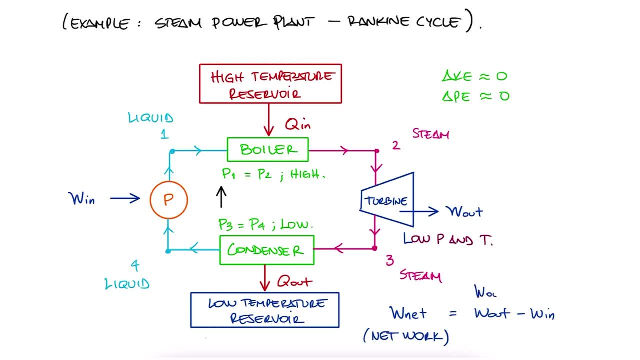 And of course, the work coming out of the turbine has to be greater than the required work to run the pump for the cycle to be worth running. Now we know that we can set our control volume to be whatever we want. So what happens if? 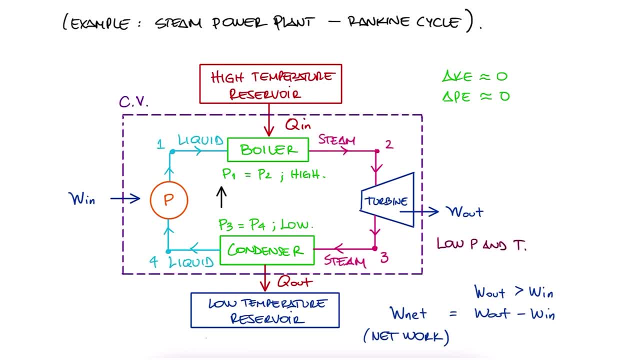 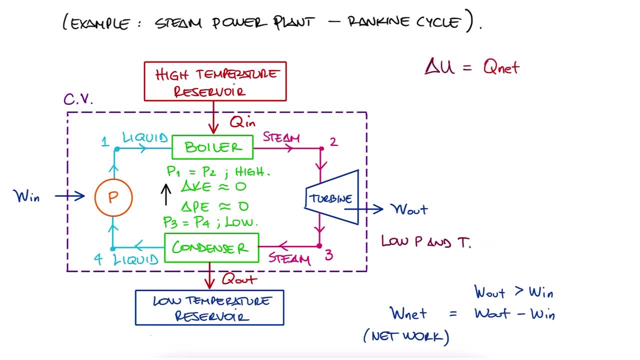 we decide our control volume encompasses the entire cycle. Well, from the first law, or energy conservation equation, we know that the change in internal energy is equal to q-net minus w-net. There is no mass coming in or out in this case, because for this control, 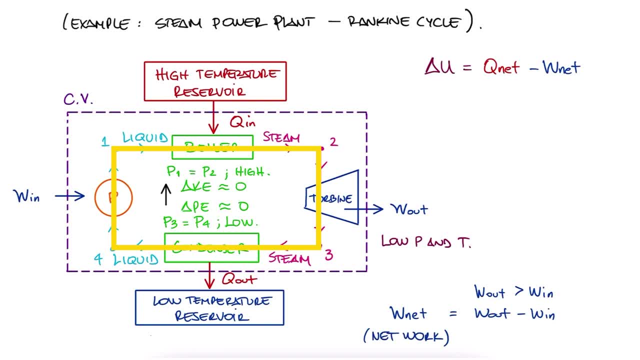 volume we selected. it is a closed system And since after one cycle the water goes from state 1 to state 1 again, the change in internal energy is zero. Therefore, the net amount of work is the same as the net amount of heat transferred Following the same sine convention. 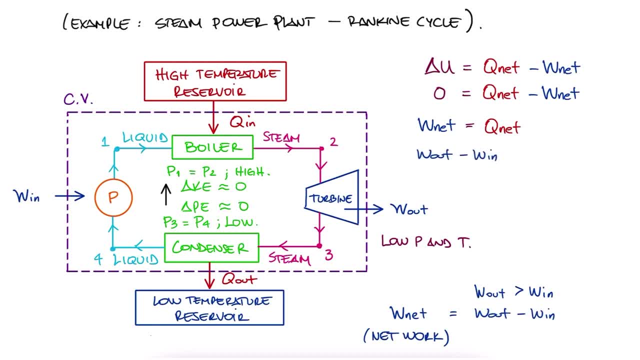 that we always use in thermo… We get the necessary control volume for every structure. This was usually the case, for our net is W out minus W in and Q net is Q in minus Q out. The efficiency of cycles like these- and this is going back to one of the first lectures of this course- which are usually